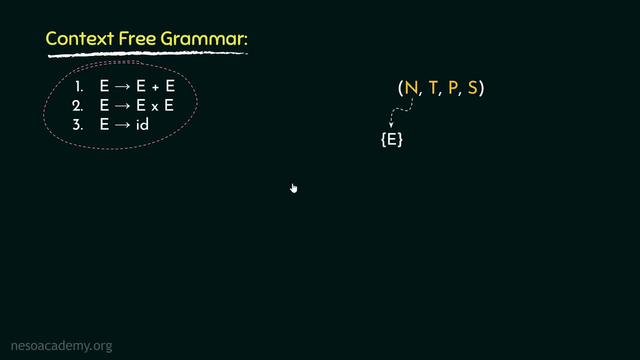 grammar. the set n contains only e. As you can observe, e is the only non-terminal here. Now t is the set containing the addition operator, the multiplication operator and id, Now p, that is, the production rule specifies all these three rules And here we have the. 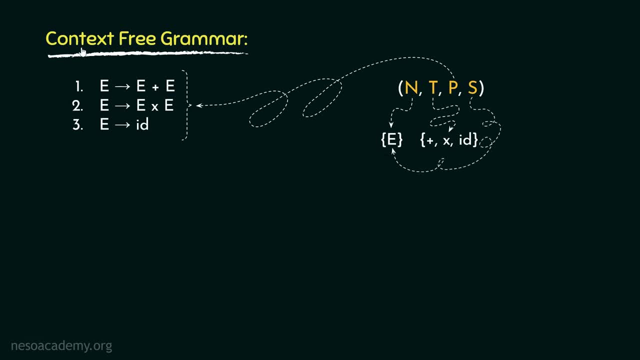 start symbol. the start symbol is e itself, So this is a grammar. Now we have claimed that this is a context-free grammar. Let's see whether that's correct. In the previous session we learned that context-free or type-2 grammar is of the form a can be rewritten. 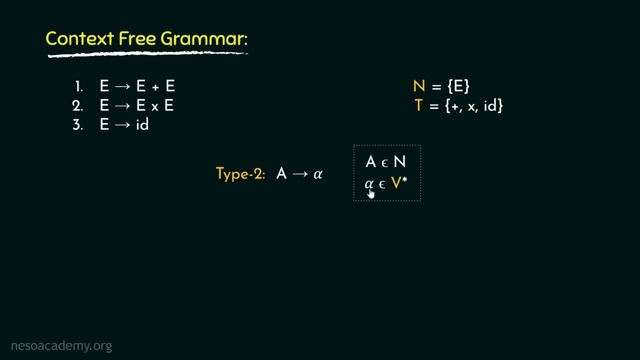 as alpha, where a belongs to n and alpha belongs to v star, which basically is any combination of non-terminals and terminals, including epsilon. Basically, the left-hand must have only one non-terminal. Well, in the LHS of all these three rules we have 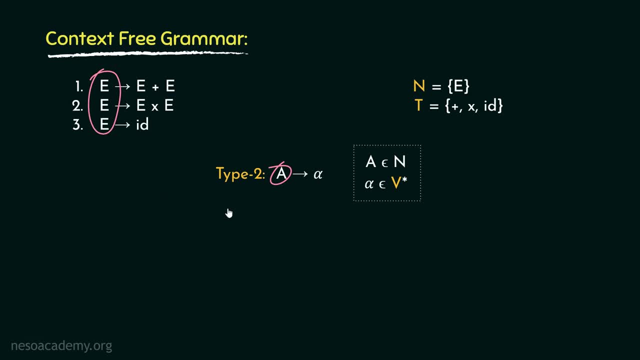 only a single non-terminal, that is e Coming to the right-hand side. the production rules are allowed to have alpha, that is, any combination of non-terminals and terminals, which is exactly the case in here as well. So now we are certain that this here is a context-free grammar. 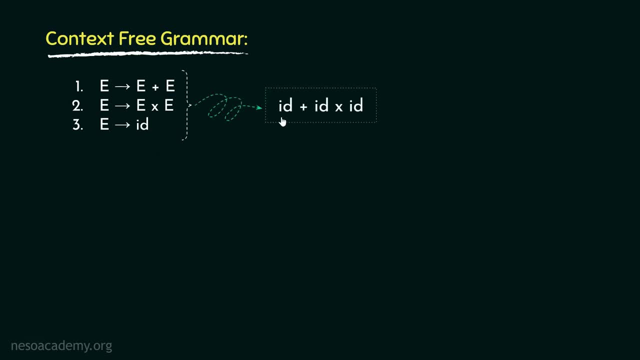 Suppose, from this we want to derive the string id plus id into id. Now there are mainly three types of derivation processes. The first one that we are about to learn is left-most derivation. So what happens in here whenever the derivation is? 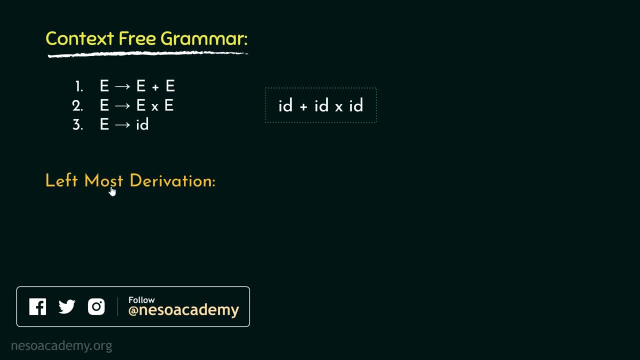 supposed to take place. we will expand the left-most non-terminal. Let me illustrate. Remember, we are to derive this string now, since the start symbol is e. only let's choose the first rule. So we state: e derives e plus e. 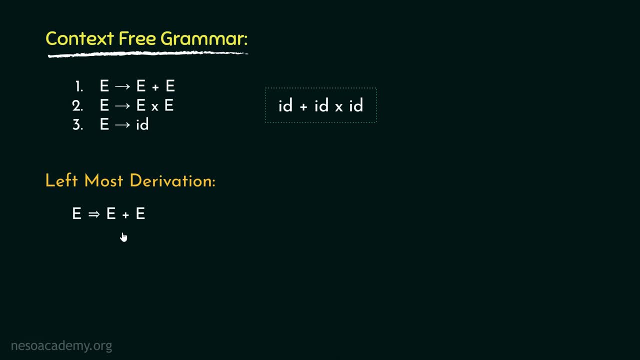 Now, since it's leftmost derivation, we will have to choose the leftmost non-terminal, that is this e for expansion. Now the final strings should be id plus id into id. Therefore, for this expansion, let's choose the rule number 3, that is, e can be written. 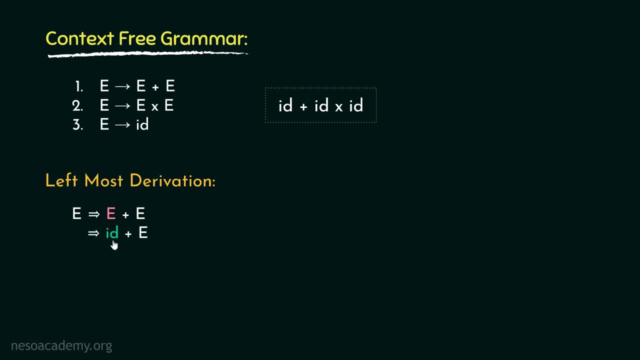 as id. So far we have covered id and plus. Now again for expansion, we will choose the leftmost variable. Observe in this sentential form, the only variable is this e. Now we want to expand this e in such a way that we can achieve this string. 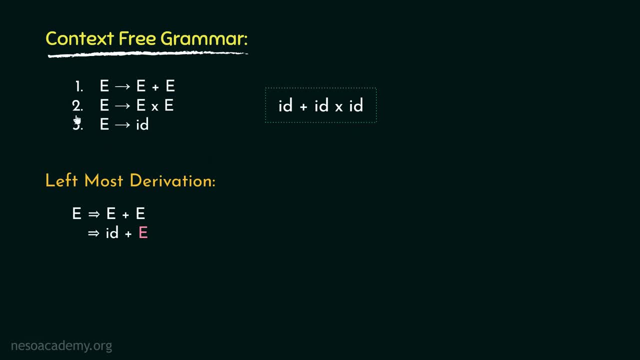 So which production rule should we choose? Yes, the second one, that is, e, can be written as e into e. So let's do that Now in this sentential form. there are two variables, and amongst them this is the leftmost. 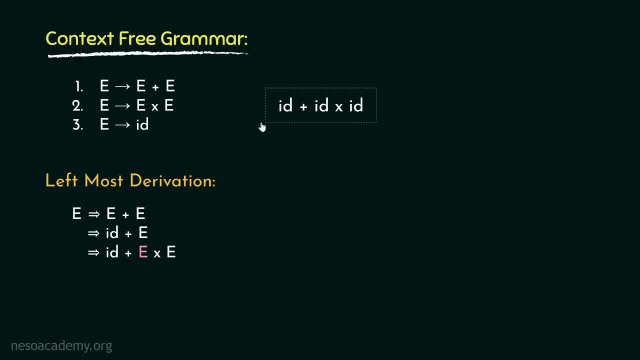 one. Now, since we already have achieved the formula, Let's choose the third rule, that is, e can be written as id. Now, this is the only e left. We will again choose the same rule for its expansion, So we derive id. 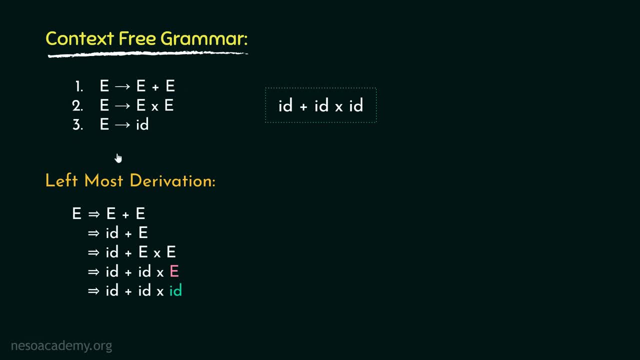 So, starting from the start symbol e, using these production rules, we finally derived the intended string, that is, id plus id, into id, And during this entire derivation process we kept on expanding the leftmost non-terminal. therefore this procedure is called leftmost derivation. 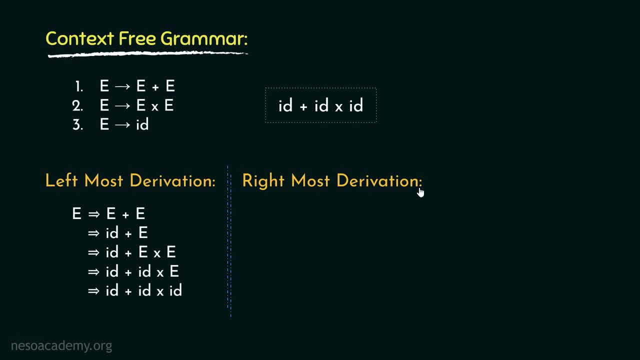 Let's now observe the next one, that is, the rightmost derivation. So from the name you already have guessed it. yes, here for expansion, we will choose the rightmost non-terminal every single time. Let's see whether we can achieve this string using rightmost derivation or not. 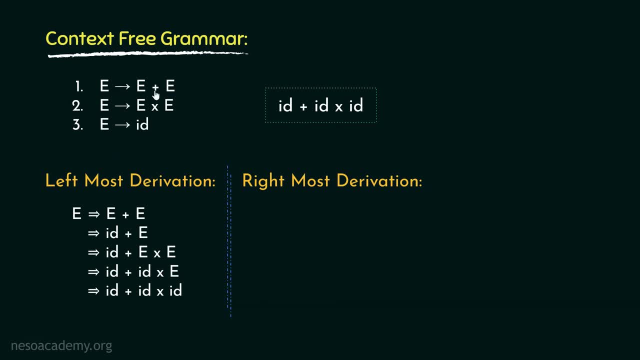 We will begin with the same rule, that is, e can be rewritten as e plus e. Therefore, we will keep on expanding e derives e plus e. Now, among these two e's, this is the rightmost non-terminal, isn't it? 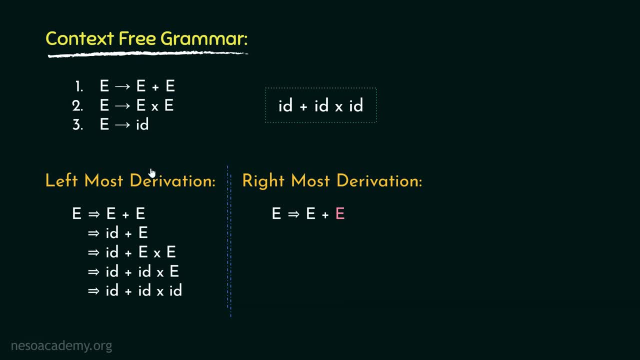 Now, in order to expand it, which rule should we choose? Observe, the string that we are supposed to achieve is id plus id into id, And we have already achieved plus and we are yet to acquire into. So let's choose the second rule. 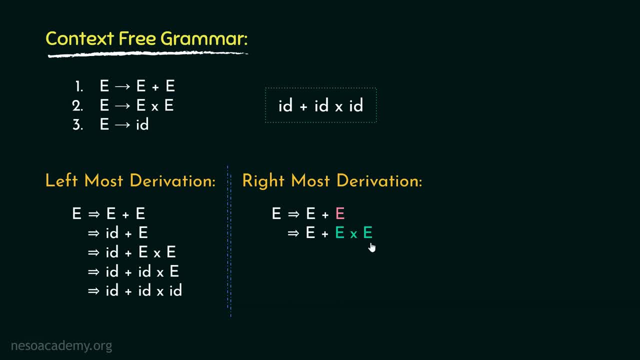 So e can be rewritten as e into e. So this form has three e's, that is, three non-terminals, And we already have achieved the format. Now this one is the rightmost non-terminal. Using the third rule, we will derive id from this one. 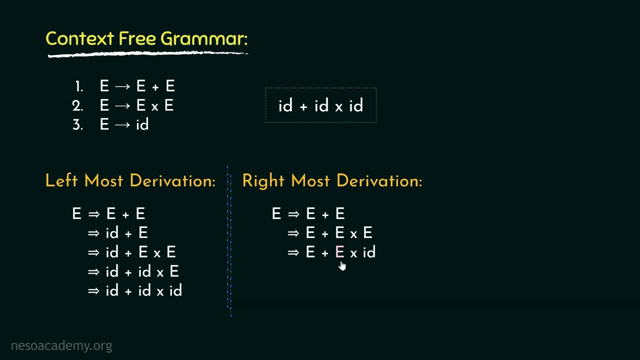 Now, among these two, this one is the rightmost one. Again, using the third production rule, we will derive id from this one. Now we have only one variable, So from this one, if we again derive id, we finally achieve the intended string. 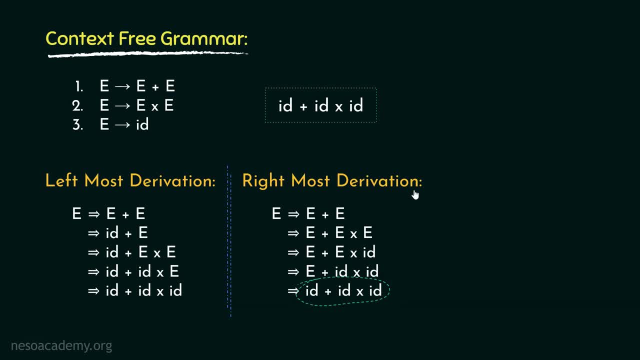 So yes, using rightmost derivation also, we derive the string id plus id into id. Here our only concern was to expand the rightmost variable during derivation. So these were the two ways. Now the next and most popular way is the parse tree derivation. 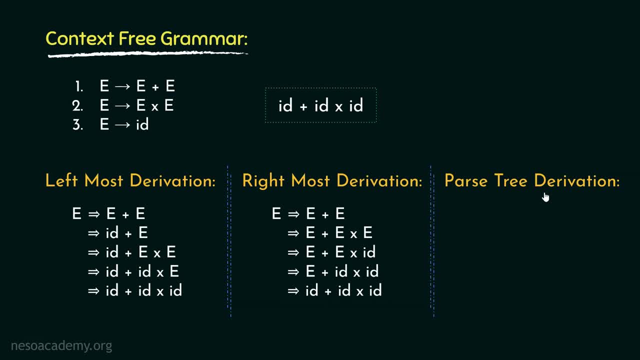 Here We can easily build the parse tree, and if our derivation is correct, then during the top to bottom, left to right traversal of the tree we will end up acquiring the string of terminal. So let's begin with the start. symbol e. 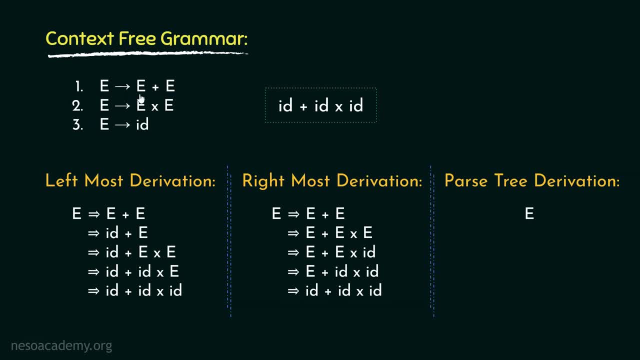 Let's choose the first rule. e can be rewritten as e plus e, So from this e we will derive e, then the addition symbol and then e. Now from this e, using the second rule, We will derive e into e. 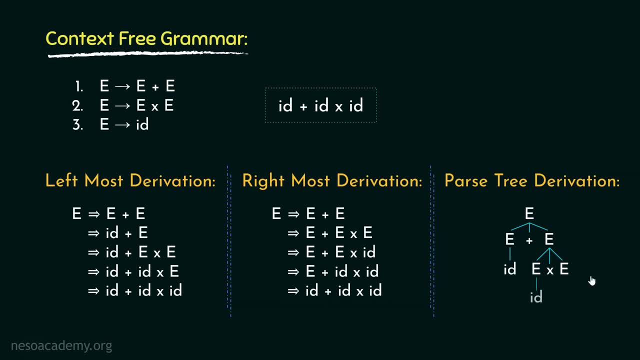 Finally, from all the three e's we will derive id using the third rule. Now let's traverse the tree, See id plus id into id. So yes, we have derived intended string using the parse tree derivation method. Do remember this is the most popular and time effective derivation procedure. 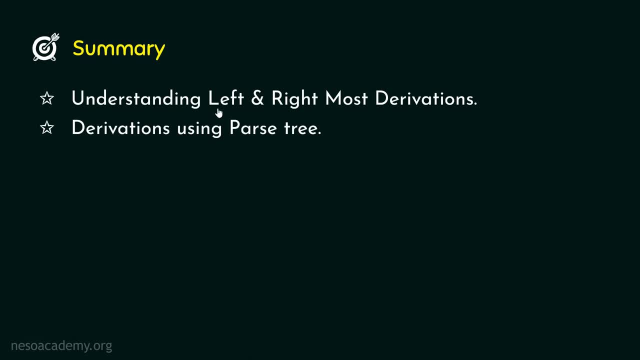 So in this session we acquired the understanding of left and right, most derivations, Also the derivation procedure using parse tree. All right, people. that will be all for this session. I hope the different derivation methods are now clear to you. In the next session we will learn about the ambiguity in context tree grammars. 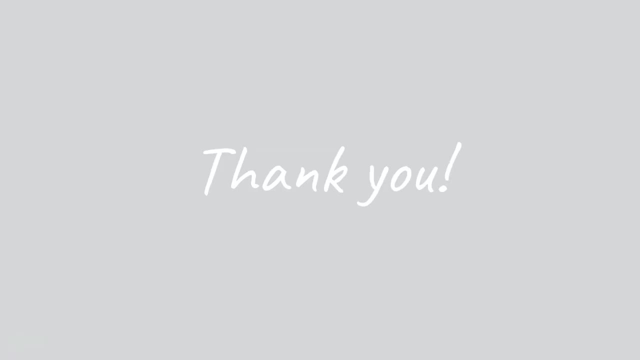 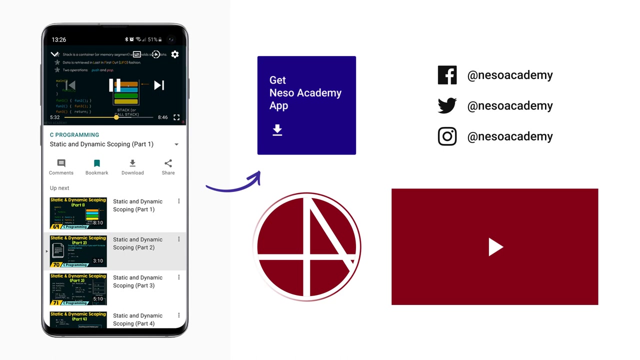 So I hope to see you in the next one. Thank you all for watching. See you in the next one.